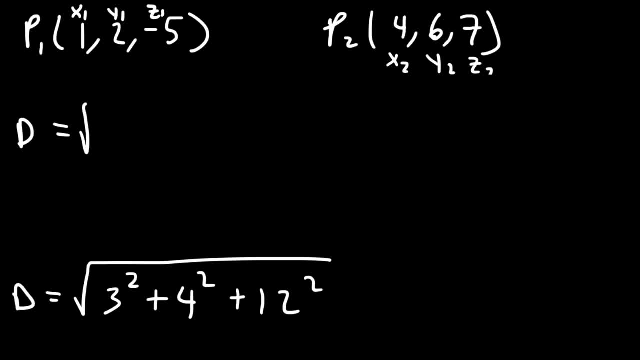 3 squared is 9,, 4 squared is 16, and 12 squared, or 12 times 12,, that's 144.. Now, 144 plus 16,, that's 160, plus 9.. So this is the square root of 169, which 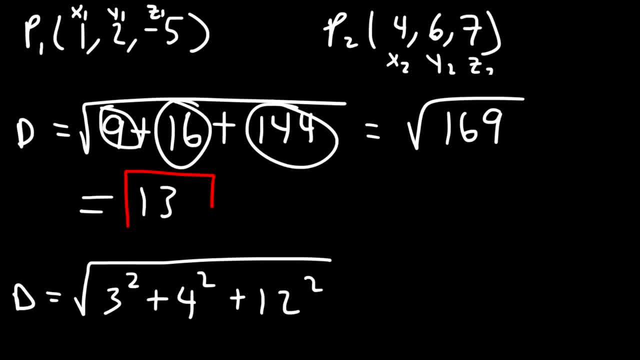 works out to be 13.. And so that's a simple way in which you could find the distance between two points in three dimensions, where you have x, y and z. Now let's plot these two points so we can understand another way in which we. 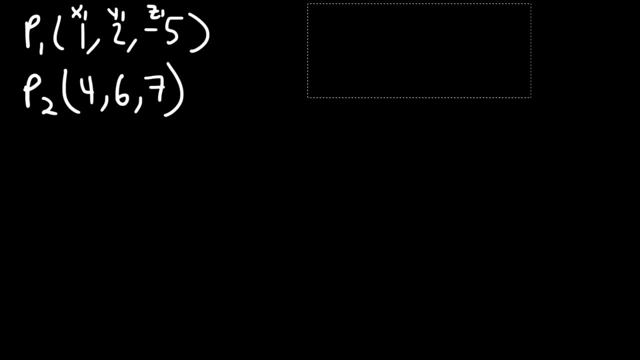 can get the answer Just to see it visually. So this is going to be the z-axis, And here we have the y-axis And this is the x-axis. Now let's begin by plotting the first point. So we have an x value of 1, and a y value of 2, and a. 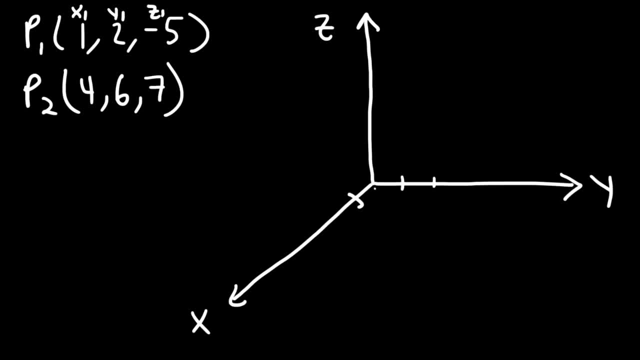 z value of negative 5.. So we need to go below, towards the negative z direction. Now, if we travel one unit along the x-axis and then draw a parallel line, the parallel dash line, along the y-axis and then starting from the point 0 to 0 on the y-axis, 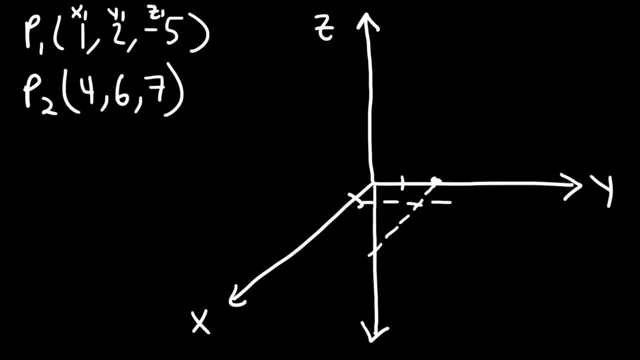 let's draw a parallel line to the x-axis, we get this point of intersection And from here what we could do is go down approximately five units along the z direction. Let's say this is 1,, 2,, 3,, 4,, 5.. 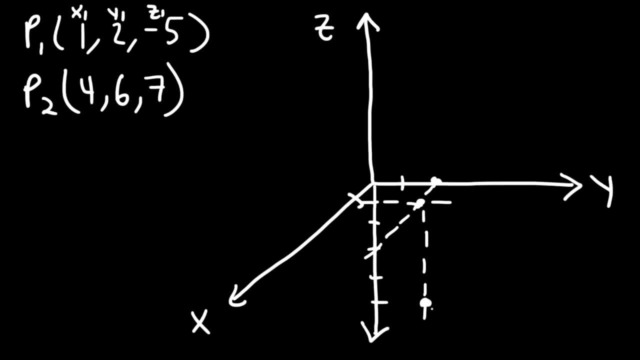 So I know it's not perfect, but let's say the point is somewhere in that region. So that would be the first point where we have an x value of 1,, a y value of 2, and a z value of negative 5.. 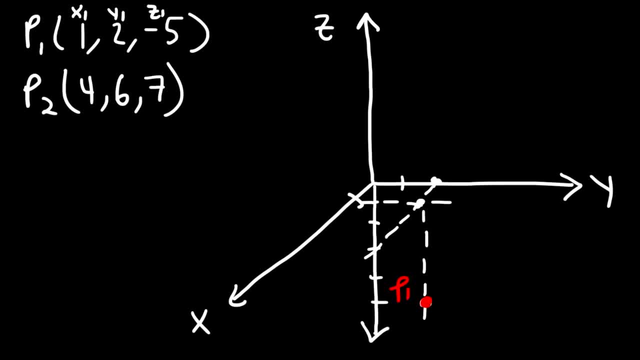 So let's call this p1.. Now let's plot the second point. So x is 4, y is 6.. So here's: 6 on the y-axis, 4 on the x-axis. Now, starting with the point on the x-axis, let's draw a dash line that's parallel to the y-axis. 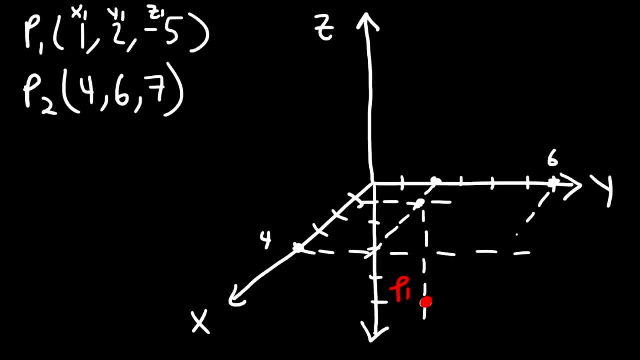 And starting with this point, let's draw a line that's parallel to the x-axis And let's highlight this point of intersection. Now, from this point, let's draw a line, or dash line, parallel to the z-axis And let's go up seven units. I'm going to ballpark it For the sake of this lesson. 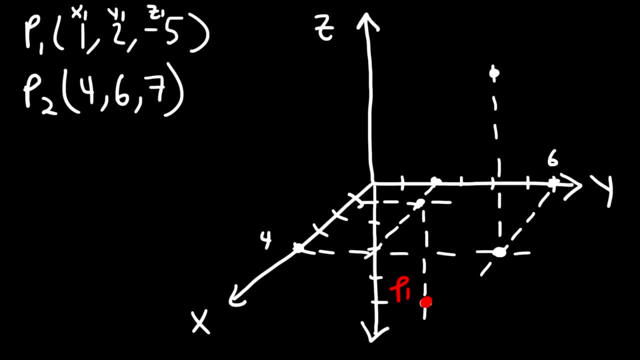 it doesn't have to be perfect for the concept that I want to teach here. So let's say that's the second point. So, as a review, we traveled four units along the x-axis And then, as you can see, six units along the y-axis. 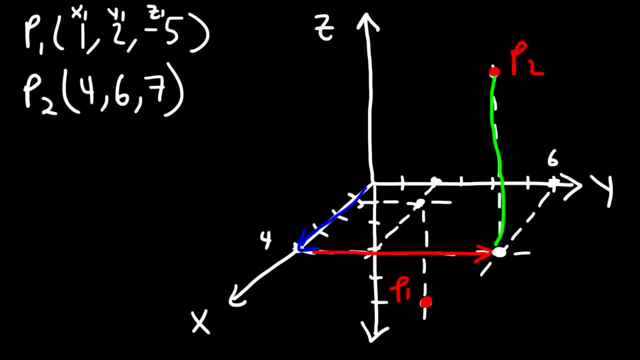 And approximately seven units along the parallel to the z-axis. Now how can we find the distance between these two points visually? We know the answer is 13,, but let's show it Now. if you look at the two points along the x-axis, we traveled. 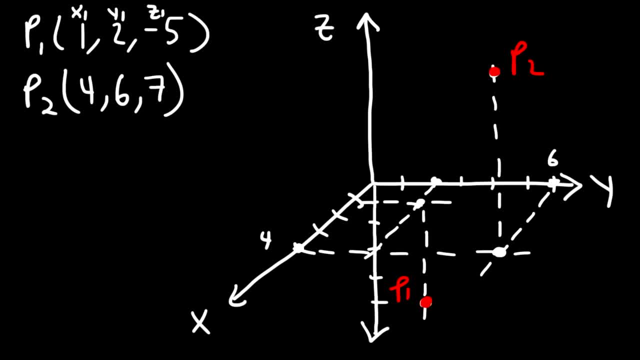 from 1 to 4.. So basically you could say that we traveled from 1 to 4.. We traveled three units this way. Now I'm running out of space, so this line is going to be pretty short. And for the y-values we went from 2 to 6. So we traveled along. 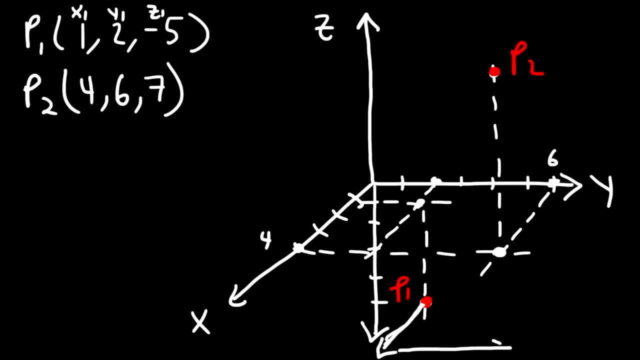 the positive y-axis You could say about four units to the right, Or rather exactly four units, not about four units. And then after that, going from negative 5 to 7, we traveled up parallel to the z-axis 12 units. 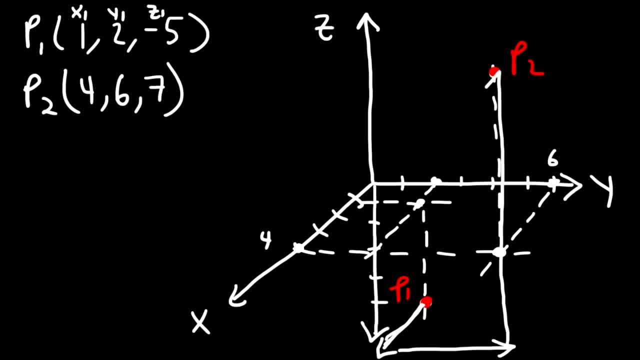 And so that will take us to this point. So let me write down these numbers. So this is 3,, 4, and 12.. Now I'm going to draw a line parallel to the y-axis and one parallel to the x-axis, And it forms a parallelogram. Now notice that this is a 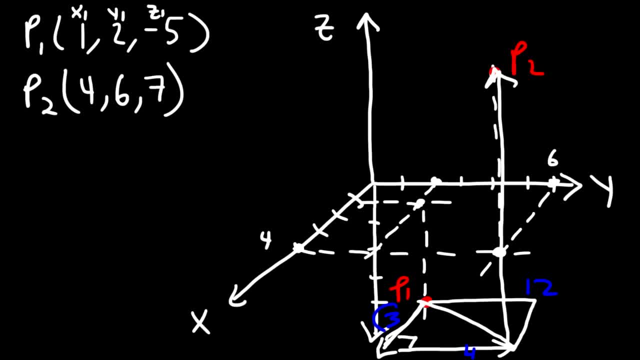 right triangle. So if this side is 3 and this side is 4, the hypotenuse of that right triangle has to be 5. based on the Pythagorean Theorem, a squared plus b squared is c squared. So 3 squared plus 4 squared is 5 squared. 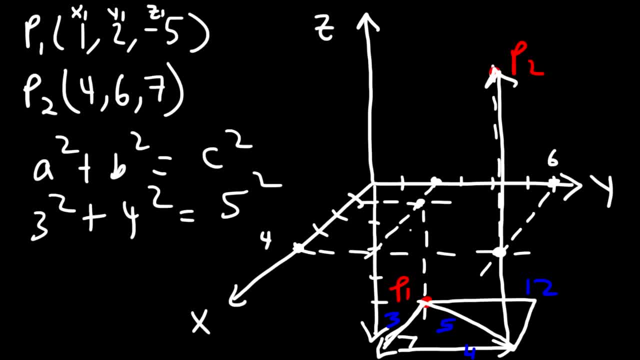 Now, what I'm going to do at this point is draw another parallelogram. So, starting with P1,, I'm going to draw a line that's parallel to the z-axis, And then another one- is 4.勆- that's parallel to this line. so notice that this XY plane that we drew is 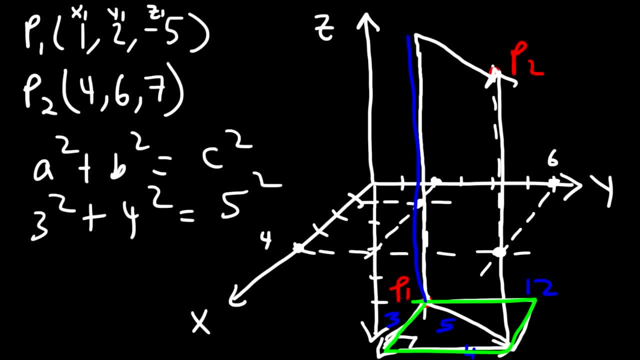 parallel- I mean not parallel, but perpendicular to this plane, and so what that means is that this is a right angle, and so if we draw the diagonal of this plane, it's going to make a right triangle, and so we're going to have a 5, 12, 13 right triangle, because 5 squared plus 12 squared is 13 squared. now let's 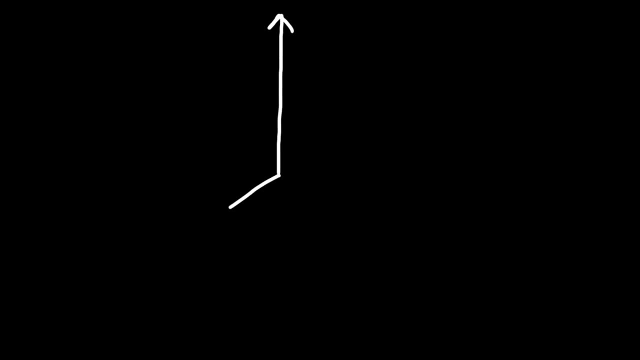 explain it using variables. so let's say the first point is the origin and we're going to travel x units, so let's just call this X and then y units, parallel to the y-axis, and then up z units, so once again we can draw a right. 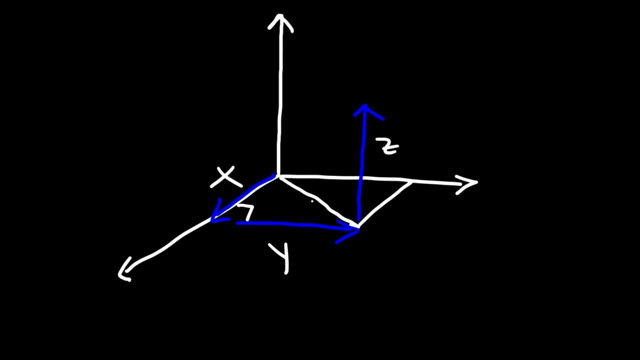 triangle and let's call this L the hypotenuse of x and y. so let's call that out, so we can say that x squared plus y squared is equal to L squared. and then we know that here is in, this is the right angle, so we can draw another triangle, and so this is going to be the 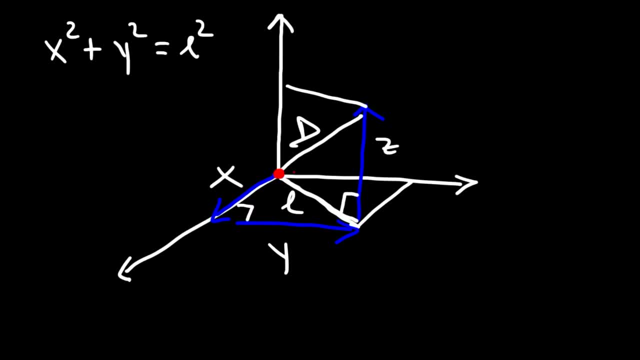 distance d between p1, which we define to be the origin, and two. So that's the distance between those two points And, as you can see, we have another right triangle between L, Z and D. So since D is the hypotenuse for that,